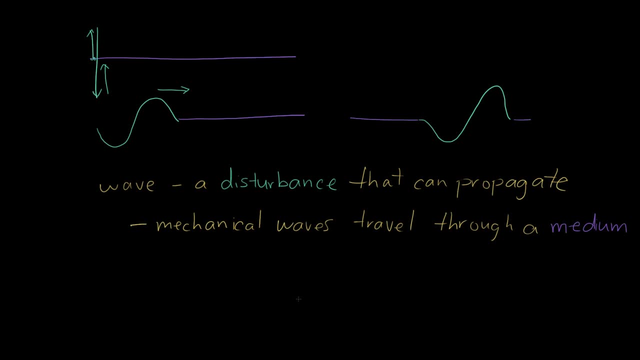 disturbance that is moving here. this squiggly shape is moving through the rope, but it isn't moving the rope to a different position. Any part of the rope might go up and down as the wave travels through that section, but the rope itself is not going anywhere. 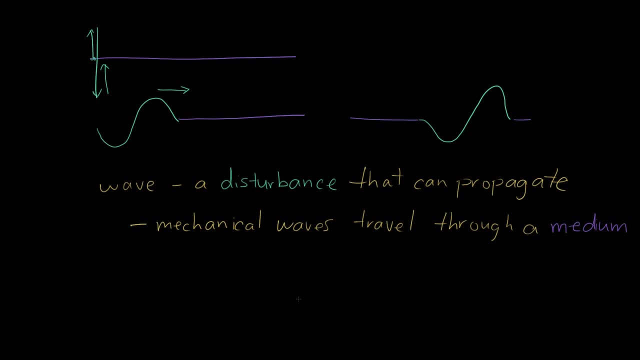 Rather, it's the kinetic energy imparted to the rope by my hand that is transferring from particle to particle and making its way through the rope. So waves transfer energy, but not matter. So in my first example, I only jerked my hand up and down once, which created a single wave. 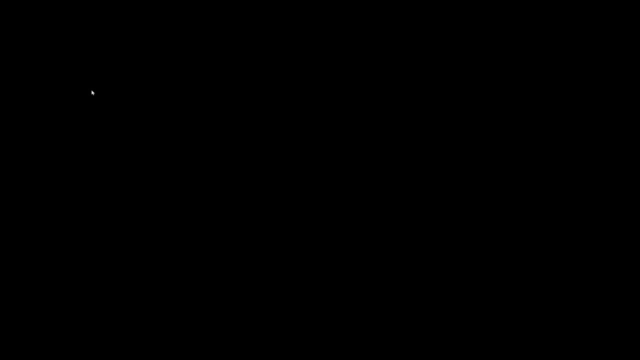 pulse that moved through my rope. If, instead, I were to keep moving my hand up and down consistently, I would see a waveform that looks something like this. And when we model a wave, there are a few key characteristics that we need to know about that wave. First is the period. Period is measured in. 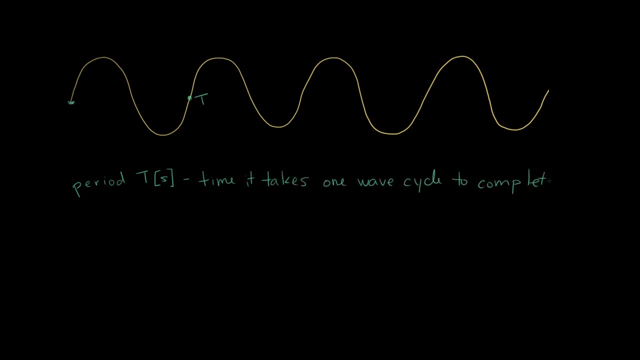 seconds, and it tells us how long it takes for one wave cycle to complete. Next is the wavelength: Measured in units of distance, like meters. the wavelength is the distance between identical points of adjacent waves. And finally, there's frequency. So if the waveform that we've drawn 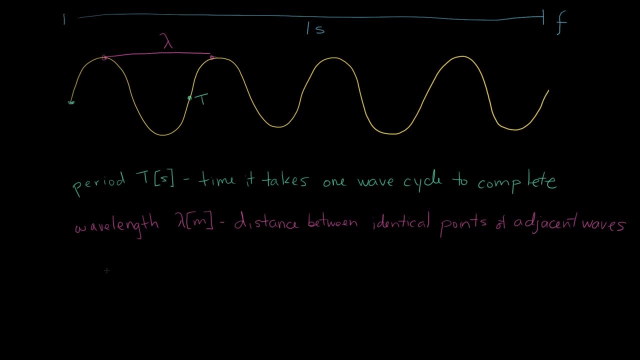 here takes one second, there are four cycles in that one second. that means it has a frequency of four hertz. So if the waveform that we've drawn here takes one second, there are four cycles in that one second. that means it has a frequency of four hertz. 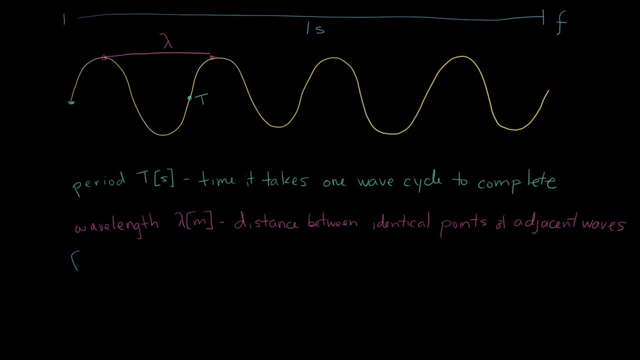 So the frequency, measured in cycles per second, tells us how many wave cycles there are every second. Now, using just these basic anatomical properties of a wave, we can start to figure out more interesting physical characteristics like speed or distance. 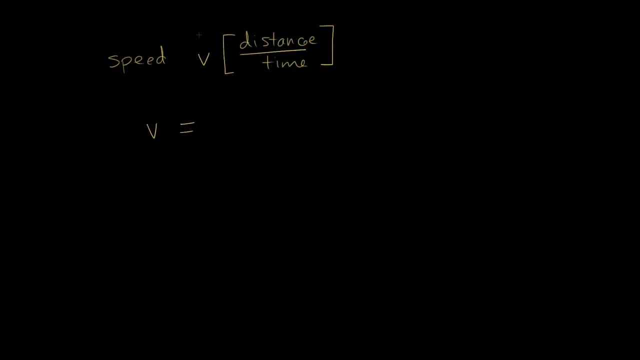 over time. If we want to know how fast a wave is traveling, we can take its wavelength, which is the distance covered by a single cycle, and multiply that by the frequency, which is how many cycles are completed in a second, a given amount of time. The cycles cancel out and we're left with units of 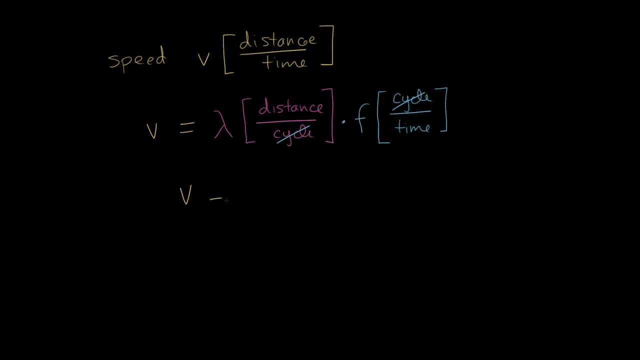 distance over time, the same as speed, And that's our equation for the speed of the wave: wavelength times, frequency: The standard units for speed are meters per second. There are a couple factors that can affect the speed of a wave. The first is the wave type, So different types of waves move at. 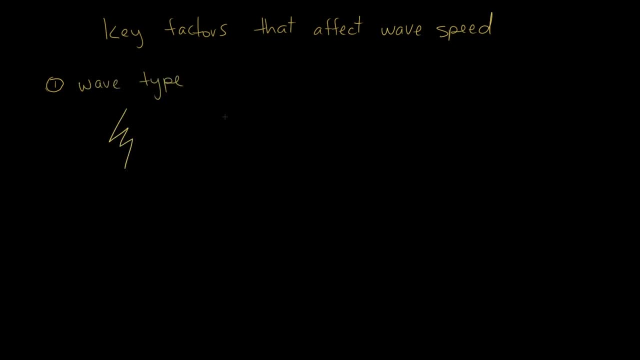 different speeds. A relatable example of different waves moving at different speeds is lightning. If you've ever seen lightning strike or been in a thunderstorm, you know that the first thing you see is the flash of lightning and then you hear the thunder associated with that lightning flash. 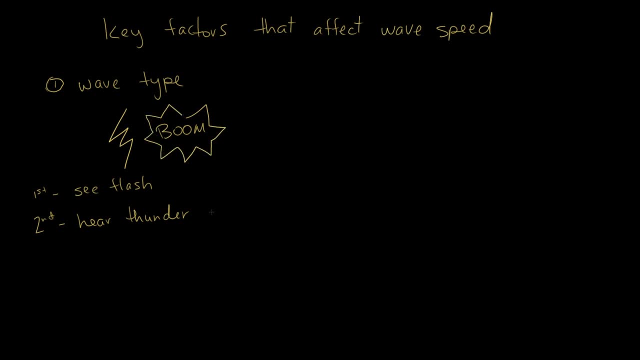 So the lightning comes first and the thunder comes second. That's because those are two different waves that are part of the same phenomenon. When the lightning strike hits, you see the flash first, because that's an electromagnetic wave- light- It travels. 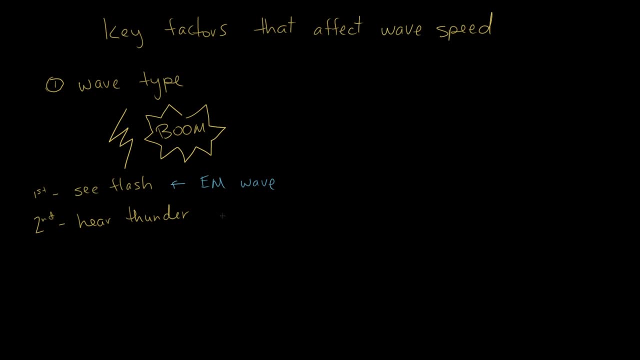 much faster than the sound associated with the lightning strike. Electromagnetic waves are special not only because they travel really fast, but they also don't need a medium to travel through. The thunder, on the other hand, is a sound wave traveling slower than the light. 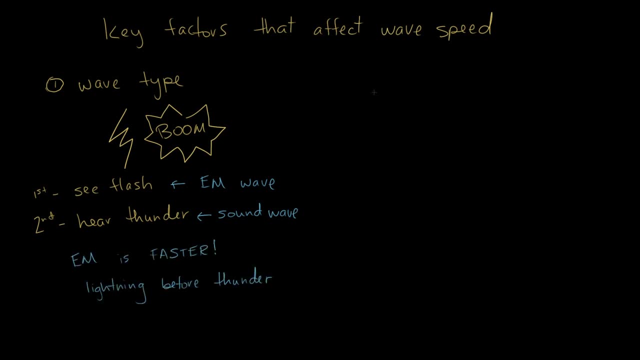 So you'll see the lightning before you hear the thunder. Different wave types move at different speeds. The second key factor that can affect the speed of a wave is the medium through which the wave travels, And we'll consider sound as an example here. So when someone is talking, 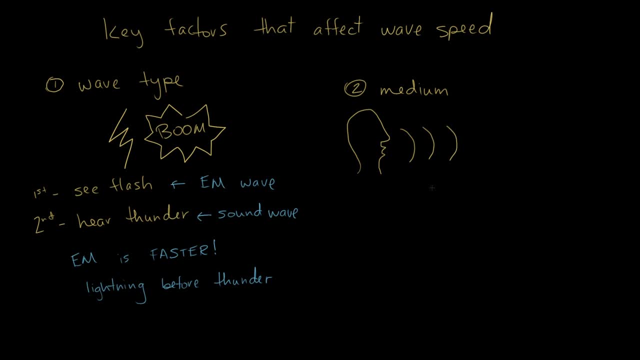 right, we have this talking head creating some vibrations of the particles and the front of their mouth. That's the sound wave, It's the vibration of those particles propagating through the air. When you speak, your vocal cords exert force on the particles just in front of you. 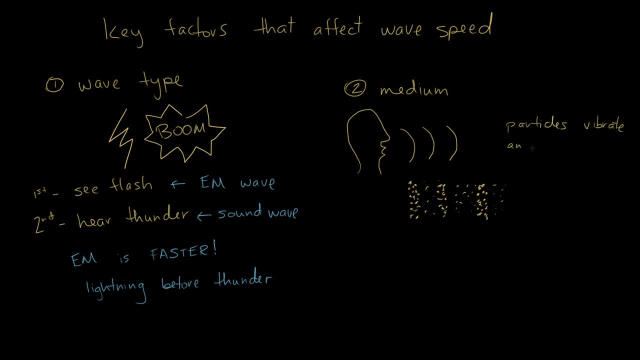 They vibrate back and forth, creating a compression that transfers to the surrounding particles. As the vibrations continue to propagate, the sound travels. You can imagine that if these particles are packed closer together, those vibrations are going to transfer a lot more quickly because the particles are colliding much faster. If you're talking about 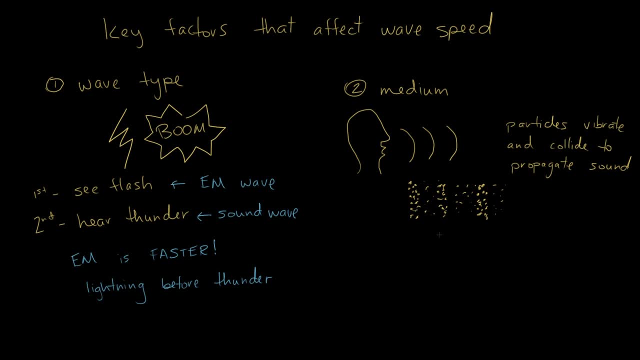 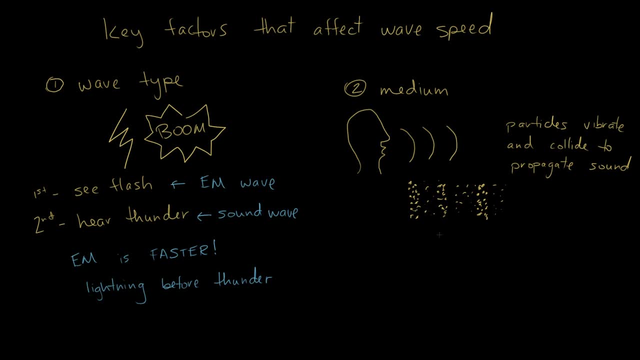 Since they're closer compacted, they collide more and the propagation of the wave happens faster. So different waves move at different speeds, and the medium through which a wave travels can also affect the speed of a wave. Alright, so let's try to summarize all this.